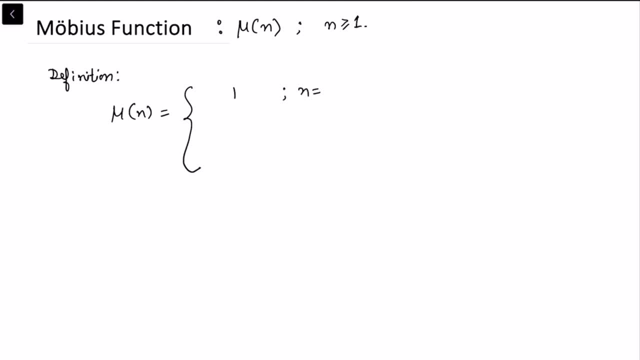 takes the value 1 if n is equal to 1.. Let's take the value 0 if it is divisible by some prime square. So whenever p is some prime and if the square of that prime divides n, this Morbius function value is 0.. This value is minus 1 to the power r if n can be written as p1, p2 up till pr. 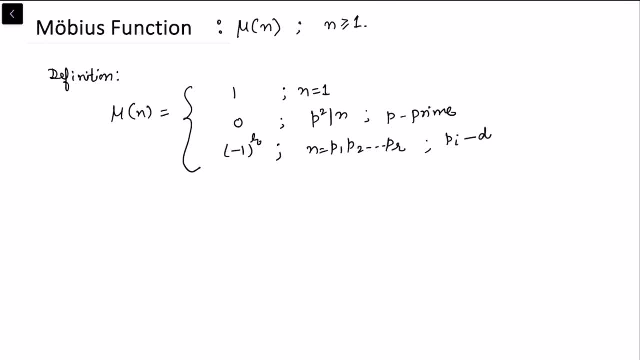 where pi's are of course distinct prime. So these are all distinct prime. so this is a prime factorization. or we can say: whenever n is not a square free number, that means p square divides n, then mu n is equal to 0.. Let's write down some of the early value: mu 1 is equal to 1 by definition. 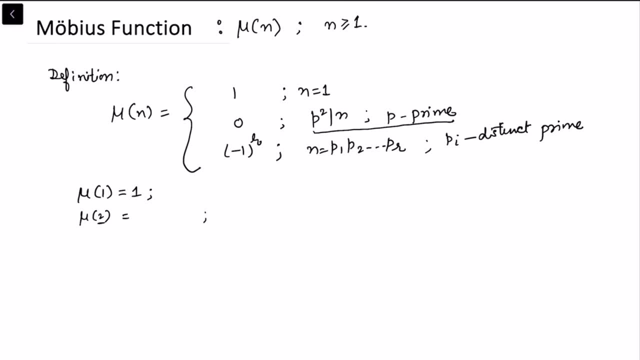 itself Mu 2, because there is only one prime here. what is the value for n when n is equal to 2.. So this is single prime and by this definition, whenever n is in the form p1, p2, this value is minus 1.. 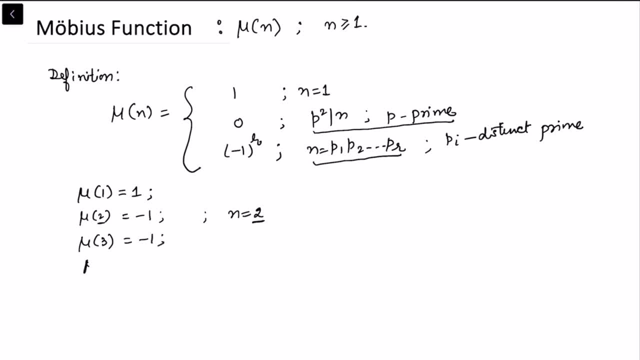 Mu 3: again this is a single prime, so this value is minus 1.. Mu 4: now 4 is actually mu of 2 square. so again now, this n is not a square free number, so this includes square and hence this value is 0.. 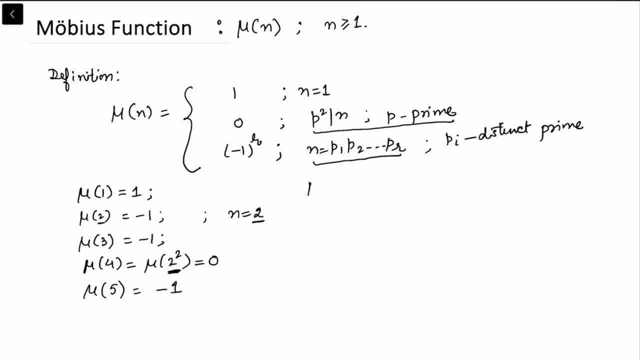 Mu 5: this is a prime, so this value is minus 1.. Mu 6: I can write down this into the prime factor. So this means I can write down n as the prime factorization of two distinct prime. Now this means it will be minus 1 to the power r, and here there are only two primes, so this is minus 1 to 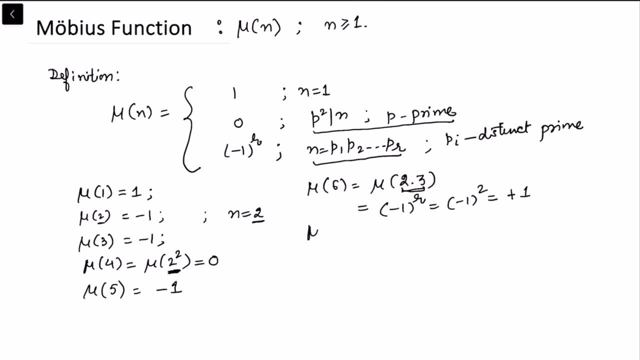 the power 2, so this will become plus 1.. Mu of 7,: 7 is a prime, so this value is minus 1.. Mu 8: again 8 is coming as 2 cube, so in 2 cube 2 square is already there, so this means 2 square, that is 4,. 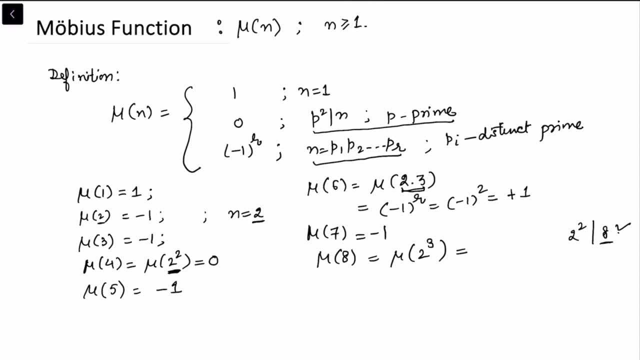 4 divides 8, so square. this 8 is not a square free number, So this value is minus 1.. So this value is 0.. Mu of 9, which is mu of 3 square, so this value is also 0.. Mu of 10, that is, mu of 2 into 5.. There. 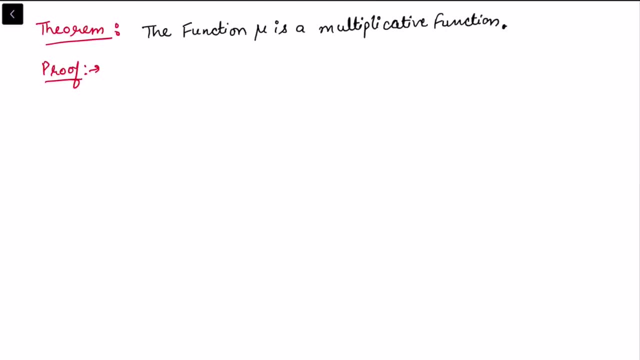 are two primes, so this value is plus 1.. The first property of the mu function is that it is a multiplicative function. So let's write down the definition for a function to be multiplicative. So this means I want to show mu of m n- this is same as mu of m- into mu of n whenever gcd of m. 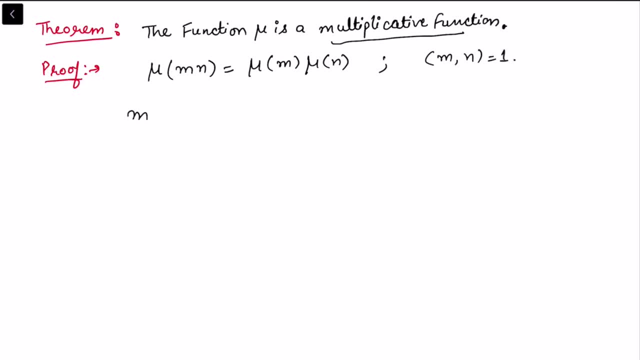 and n is equal to 1.. So let's consider m and n in a general form. Let me to take m into the prime factorization p1, p2 up till pr, and let's take the n also, prime factorization q1, q2 up till some q times, s and. 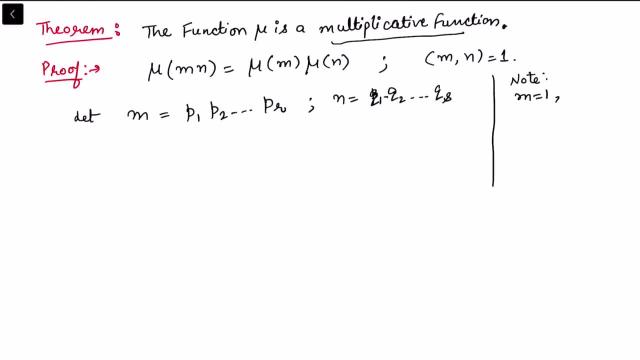 notice that whenever m and n is equal to 1, both of them are equal to 1.. So this means mu of m n. this is same as mu of m into mu of n, because mu of 1 the product is 1, 1 into 1, and here also. 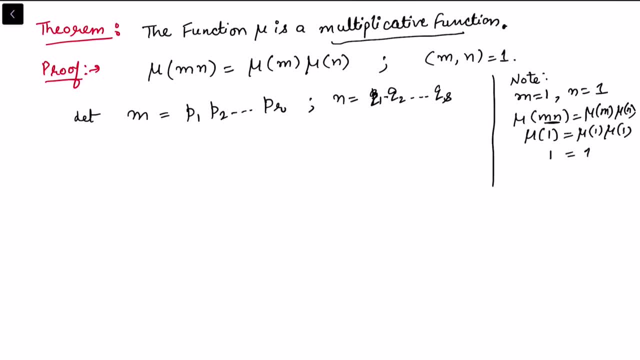 this is mu 1 into mu 1.. So both sides. this is trivially true, So there is nothing new to prove. whenever m is equal to 1 and n is equal to 1.. Whenever there is a prime square that divides m, in this case mu m will be 0. or we say: whenever there is a prime square that divides n, so mu n. 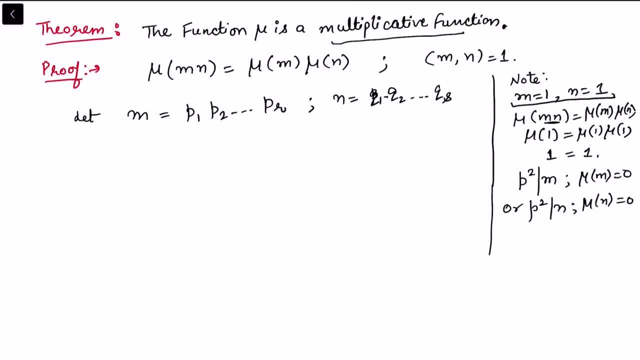 will be 0. So we will leave this case whenever there is a square involved in those prime factorization of m and n. So because of the property that whenever these m and n are not square, free numbers, so this value will be 0. So, excluding 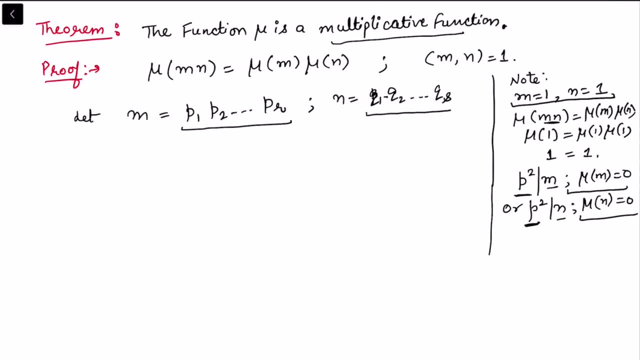 these case. now I consider m in the prime factorization, where each prime appear with the power only 1.. Now I want to prove mu of m, n. So let's just substitute these values: m is p1, p2 up till pr. these are distinct primes. and of course n is q1 up till qs. So just take the multiplication. 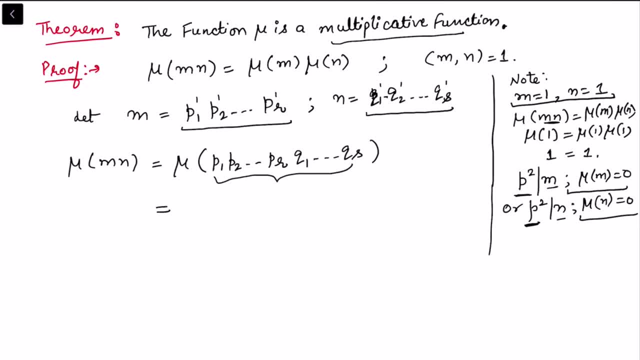 of m? n and here, how many total prime do we have inside? we have r plus s primes, So this is same as minus 1 to the power of n. So we have r plus s primes, So this is same as minus 1 to the power. 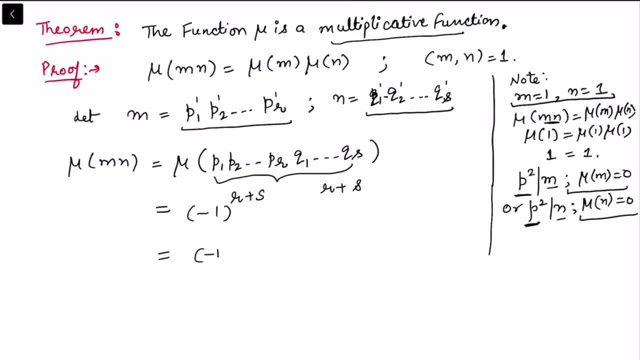 r plus s. by definition, This is same as minus 1 to the power r into minus 1 to the power s. This I can write it as mu of p1 up till pr into mu of q1 up till qs, because by definition minus. 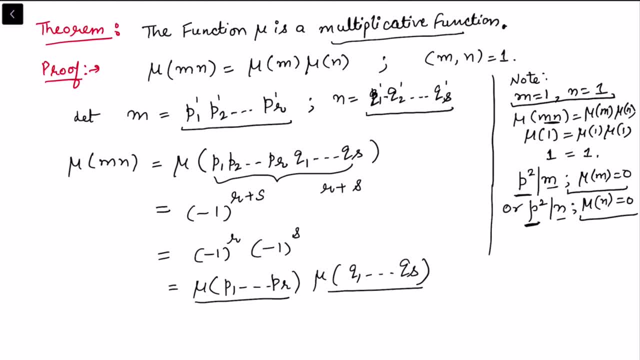 1 to the power r can be written into this form. minus 1 s to the power s can be written into this form. This is same as mu of m into mu of n, and hence the result that Moebius function is a multiplicative function. So now in this theorem we: 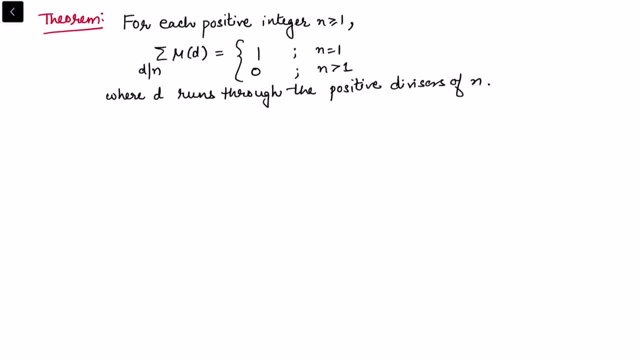 want to prove that, for each positive integer, n greater than or equal to 1, summation of mu d, where d divides n and d runs through the positive divisors of n, This is equal to 1 or 0 when n is equal to 1 and n strictly greater than 1.. Now let's prove this case, and in this case I want to run. 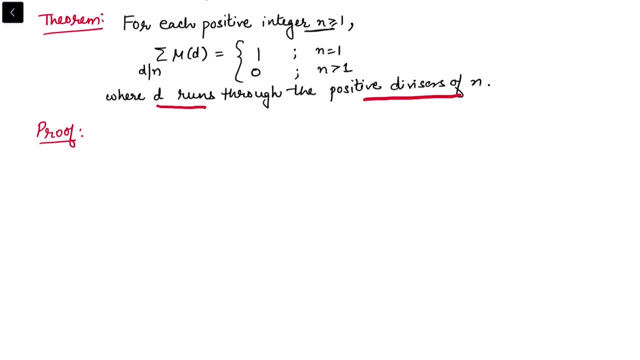 over all divisor over the positive integer n. So let us consider the prime factorization of n. So n has a prime factorization in this form: p1 to the power, k1, up till so on, pr to the power kr. and let's take summation: mu d d divides n as capital F of n, and we are just 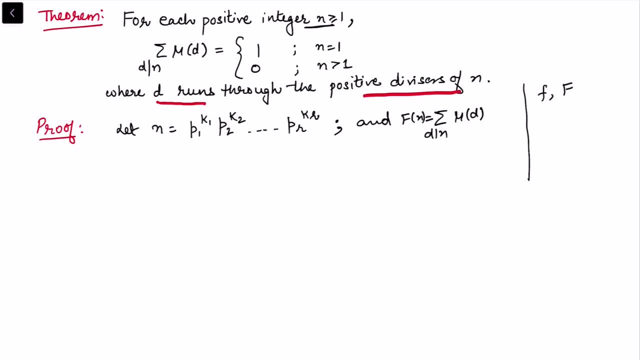 using now this result that if small f and capital F are two arithmetic function and capital F of n is related to small f, s in this formula d divides n, Then if small f is multiplicative, this is multiplicative. then that implies that capital F is also multiplicative. So we just have proved that. 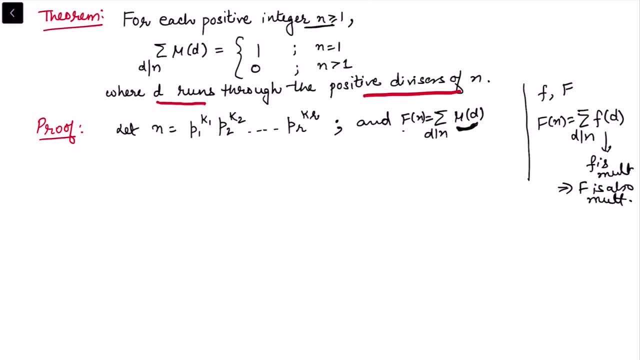 mu d is a multiplicative. If mu d is a multiplicative function, then capital F is also multiplicative function. So if I can now write capital F of n, this will become F of p1 to the power k1, up till so on. just substitute the. 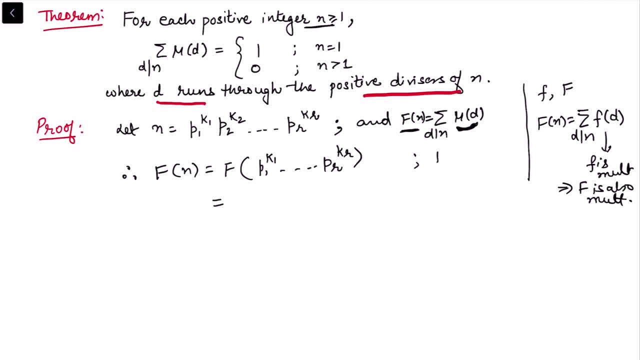 value of n. and because now F is multiplicative- we have just said that F is multiplicative function- this means this is same as F of p1 to the power k1 and so on, F of pr to the power kr. Now I am just interested in knowing. so what is F of p1 to the power k1 and what is F of pr to the power kr? 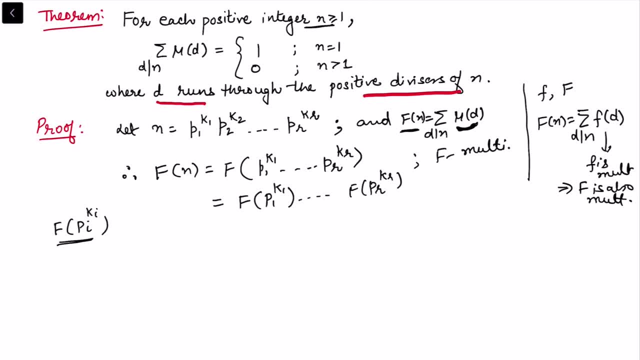 If I know now this value, then I can just substitute into this above expression and I can find out. So now let us see what is this case. So we want to now find this expression and now, by the definition that we have given here to Fn function, let's now write it as F of pi to the power ki. this is equal. 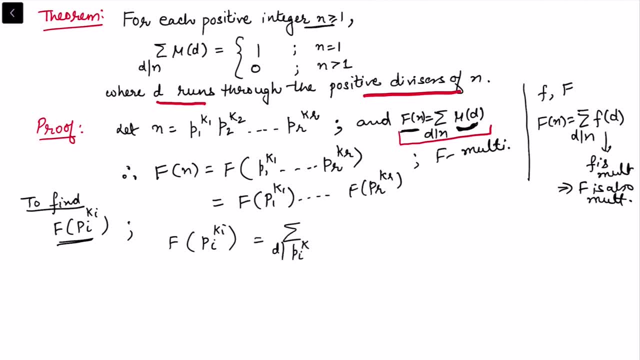 to summation. d divides pi to the power ki. this is now taking the value n, and then we have mu of d. So d is the divisor. d is divisor of pi to the power ki. Now, what are the divisors of pi to the power ki? this is one is divisor of every number. so one will come here. then we have pi, then we'll. 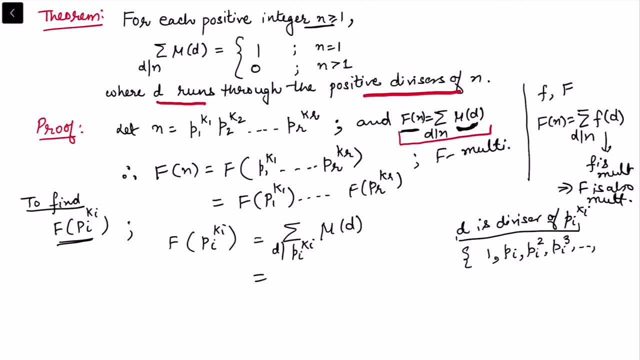 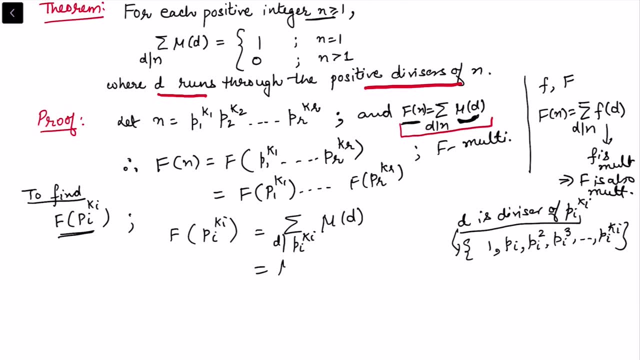 have pi square, pi cube, and so on, up till pi, to the power ki. So these are the values that has been taken by d. So substitute these value, say when d is equal to 1. so this is summation. so I then I'll take the second divisor. this is mu of pi plus, mu of pi square plus on. consider all the. 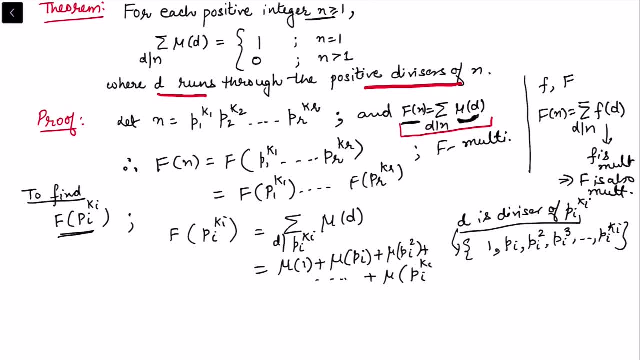 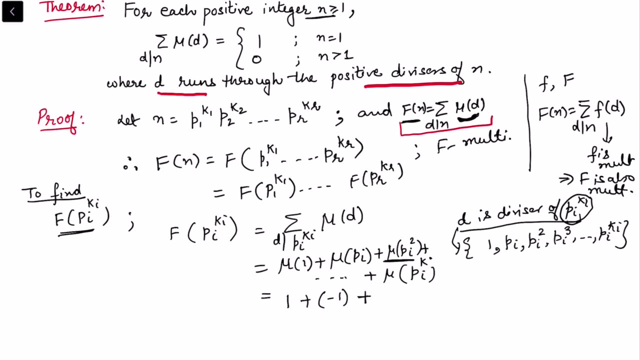 divisors. till last divisor is pi to the power ki, because here this expression is pi to the power ki. Now we know mu value is 1, mu of pi value is minus 1, plus all these term and this expression: mu i pi square, because it is a square. so this value is 0 and hence similarly other all. 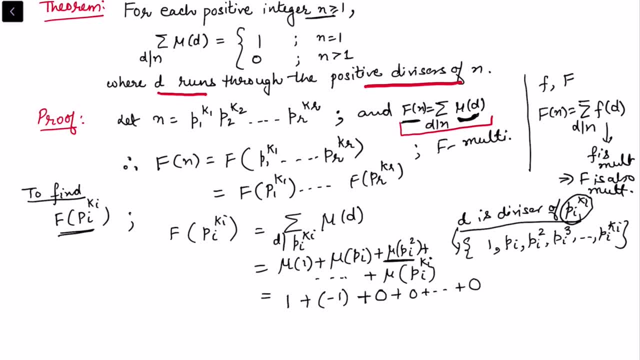 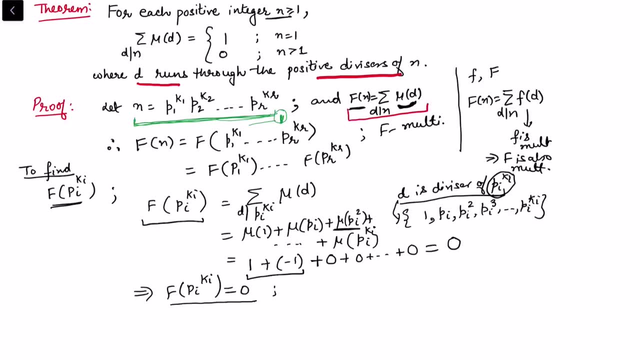 quantities. where there is a power which is larger than 2, all quantities are 0. So now this 1 minus 1, this value is also 0. So this implies f of pi to the power. ki is 0 for n strictly greater than 1 whenever we have a prime factorization. that I have now denoted by equation number. 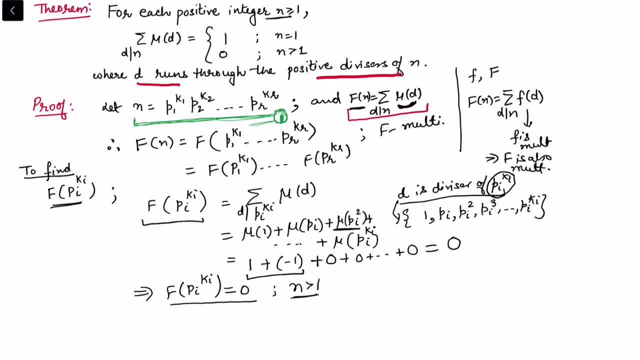 1.. Now this means now you substitute here this expression: f of p1, k1 is 0, f of p2, k2 is 0, because this number is 0 for every i, So this whole expression is 0.. Now suppose that if my n is 1, okay, suppose if n is 1, in that case, when n is equal to 1, so in 1 in. 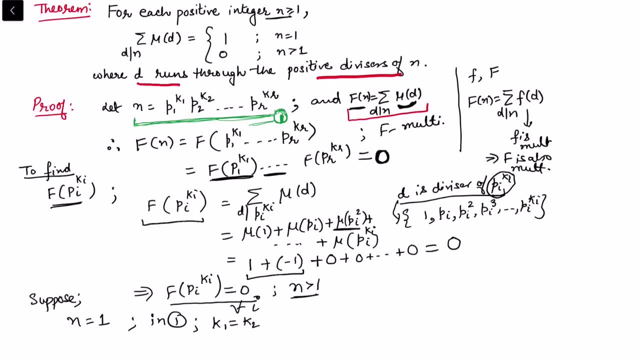 equation number 1. the only possibility is that k1, k2, all these power of the primes are equal to 0. In that case n will take the value 1 only, because anything raised to power 0 will make this quantity as 1, and in this case capital f of n. this is same as summation d.